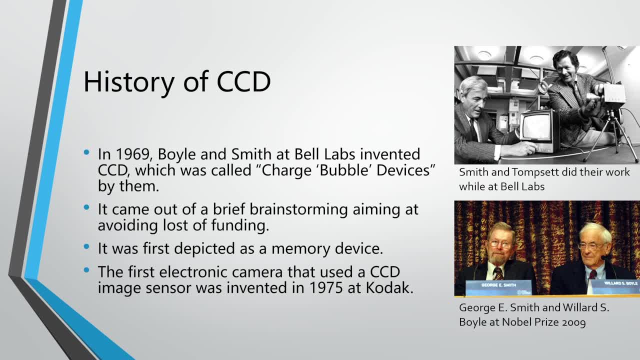 Bell Labs, Smith and Boyle also won the Nobel Prize in 2009 because of the invention. The first electronic camera that used the CCD image sensor was invented in 1975 at Kodak, but we know that Kodak filed for bankruptcy this year, probably because, even though they invented, 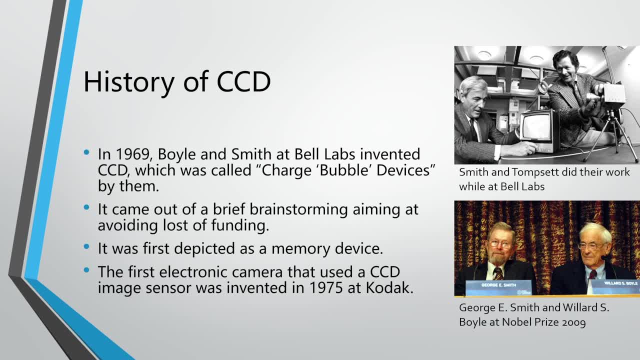 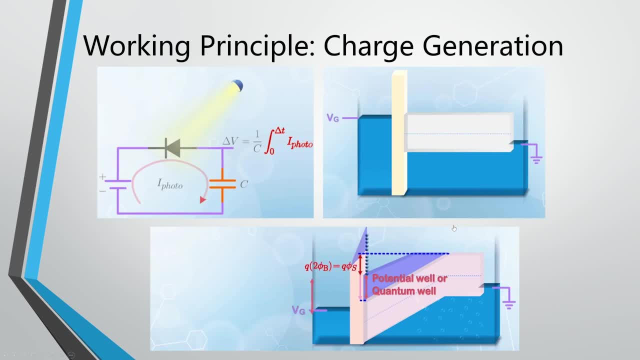 the first camera, they didn't realize how influential it could be by still focusing on the film business. From the photoelectric effect. we know that if we shine light on semiconductor we promote electrons from convalescence band to conduction band. However, that cannot separate. 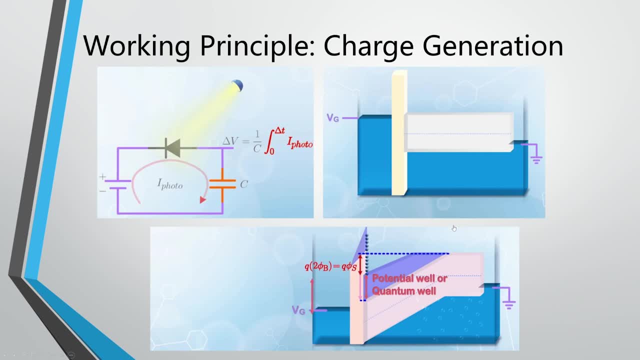 holes and electrons and they will finally recombine. If the light is shining on a p-n junction, electrons will move to one side and holes to another side. Current is generated, Then we put a capacitor Next to it which acts as an integrator. charges accumulate as a capacitor to indicate the light. 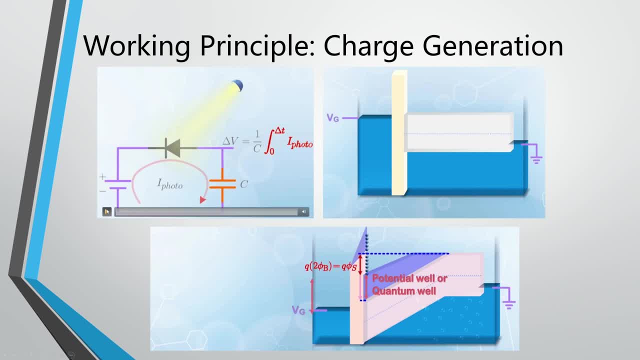 intensity. This forms MOS capacitor, which stands for metal oxide silicon. If a fast DC voltage is applied to the gate terminal higher than the threshold voltage, we break the thermal equilibrium and deplete holes further away than this maximum distance called deep depletion mode. Thermal equilibrium can be simply understood. 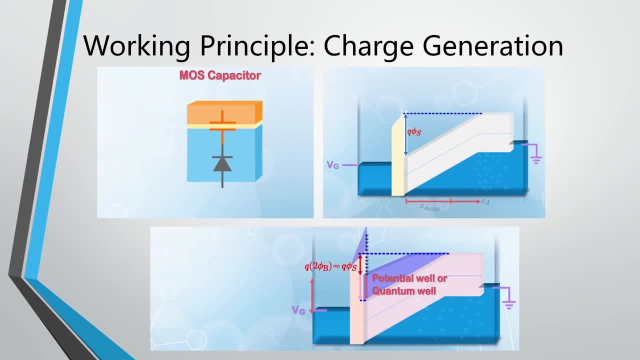 as aczypleλι oneselfsedeisch мне são duas questões Sca Per playback. nós temos uma sequência de carga igual do volcano de as Provosto, que também está sendo utilizado quando llevamos charge ao saldo. This is information paper thatpelsoasser. 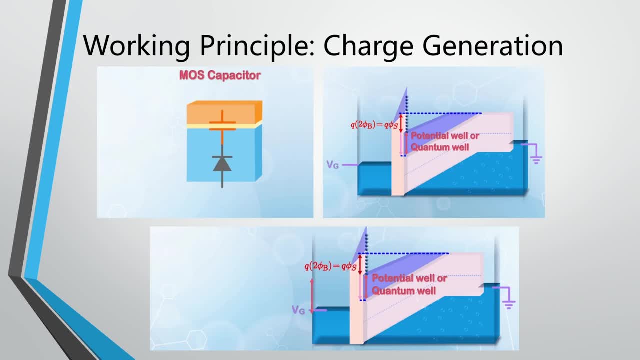 The state is higher than it is. Just as In divorced operations, A quantum well is formed. We can make an analogy of the quantum well as a water well. The soil has holes inside to store the underground water. If we dig a well and let time pass, 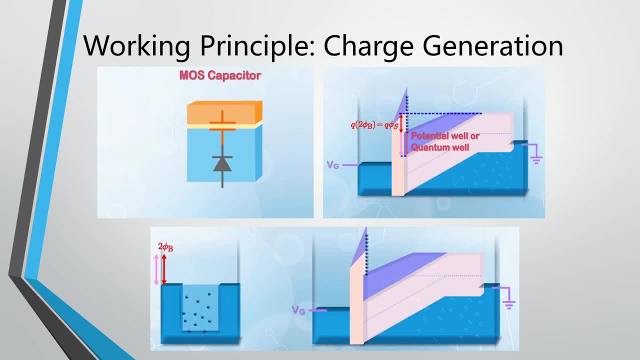 underground water will finally come out of it and fill the water. The volume of the well is determined by the gate voltage and capacitance of oxide. After the well is created, we shine light on it and charges accumulate, just like raining on the well and water accumulates in. 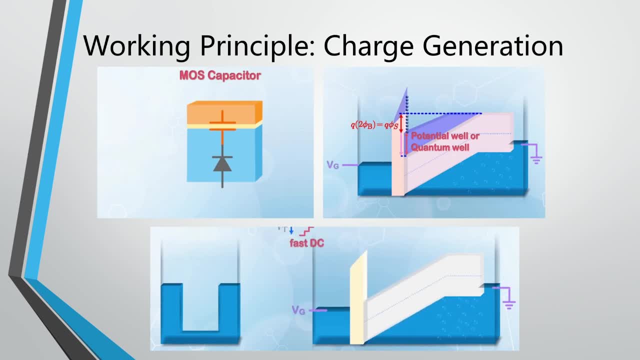 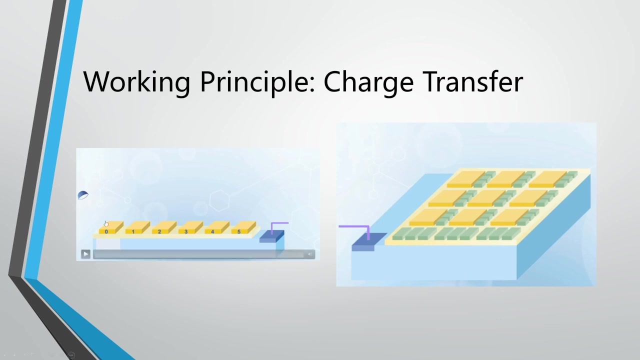 the well. If we drain the water out of the well and measure its amount quickly, before underground water comes out and affects the measurement, we can know the intensity of the rain just like the intensity of the light. After we have charges, we need to transfer them. We put several CCD together and put a. 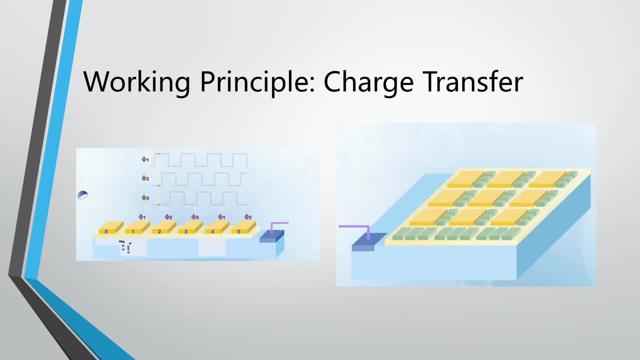 phase shift clock on the gate. This is why it is called charge coupled device. Only number zero is shined by light, while others are covered by metal. in order to maintain the number of charges during transfer, At the end of transfer the number of charges is read out by a charge to voltage circuit. 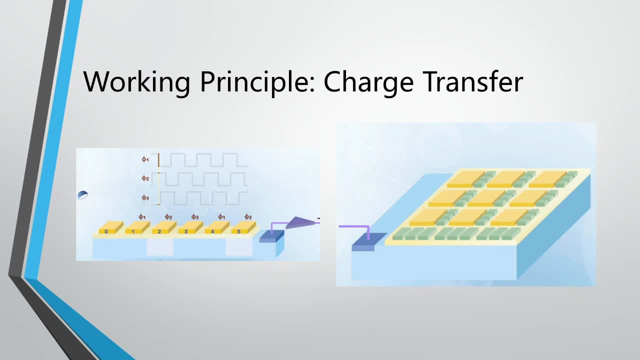 We can see that it can act as a shift register, While the storage in the register is the number of charges. This is a 1D situation, but to form imaging sensors, we make it into an array, as shown at right, In order to save space. 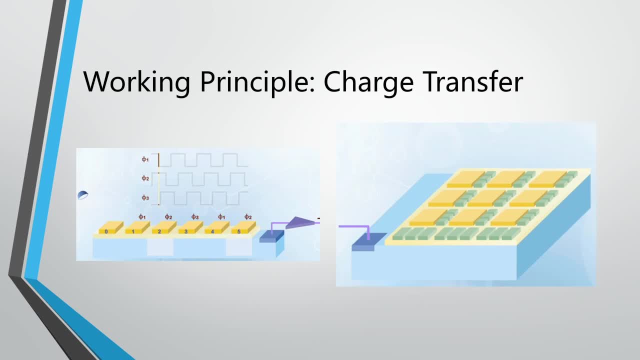 we make the green CCD from number one to number five very small, while keeping the yellow number zero big. However, in order to maintain the depth of the well, a high gate voltage is needed. All the charges in each pixel are read out one by one by the same charge. 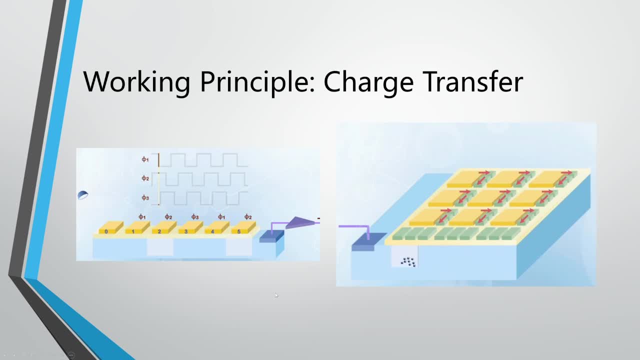 circuit. All the charges in each pixel are read out one by one by the same charge circuit. After forming the array, we need two more things to make it an imaging sensor: Microlens are used to concentrate the light on the wells- and green, red and blue color filters that form Bayer. 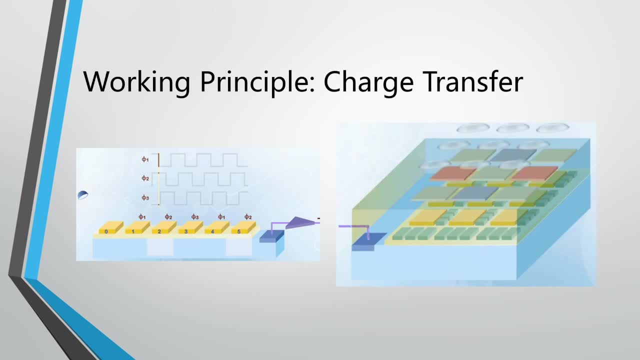 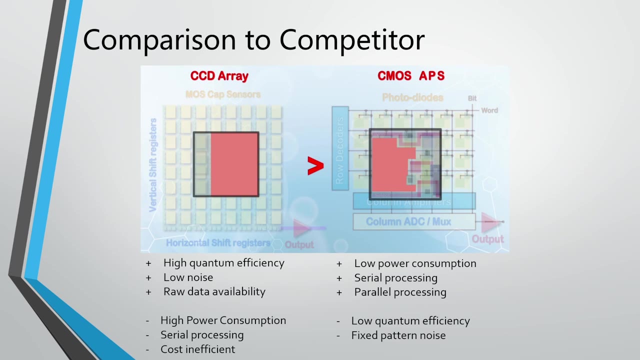 patterns are used to distinguish the color of lights. Nowadays the biggest competitor of CCD arrays is the CMOS APS. The CMOS APS doesn't need a potential well to store the charges, because they are converted to voltage at the pixel. The generated charges cannot drive the loading capacitance in. 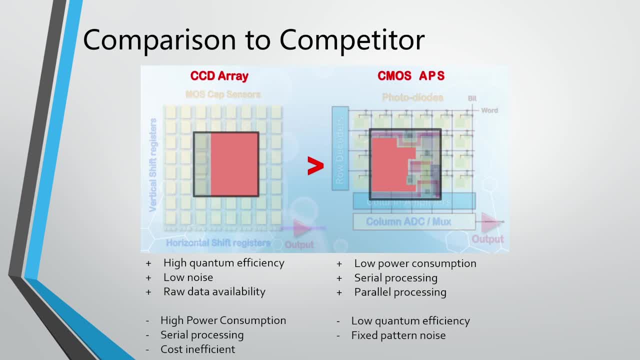 the charge-to-voltage circuit. Therefore, an amplifier is needed at each pixel. It is not possible at early days due to large transistor size. However, even nowadays the amplifier still takes some space in the CMOS APS. Therefore the quite 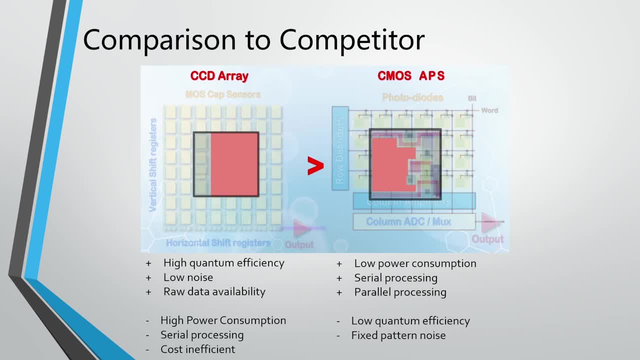 an efficiency in the CCD array is higher than the CMOS because we can see the pink area that can convert the photon to the electron is larger than the percentage in CMOS. CCD array also have no noise compared to CMOS because every charges are measured by the same. 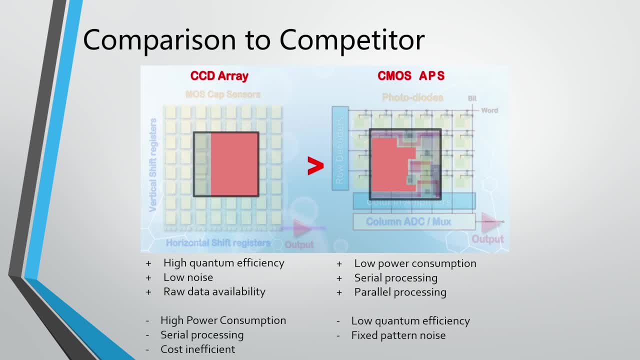 circuits. However, in CMOS, because we have an amplifier and converter in each pixel, we will have a fixed pattern noise. The raw data is also available in CCD because the charges are read out and the data we get is the number of charges. However, in CMOS, all we know is the voltage that was converted. 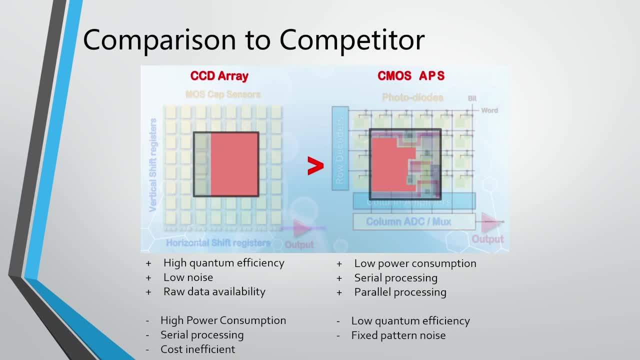 There are also some disadvantages in CCD. The high power consumption is because of the high voltage that we need to create the quantum. well, Serial processing in CCD array also make it process in CMOS, because in CMOS all the data are converted simultaneously with all the amplifiers. 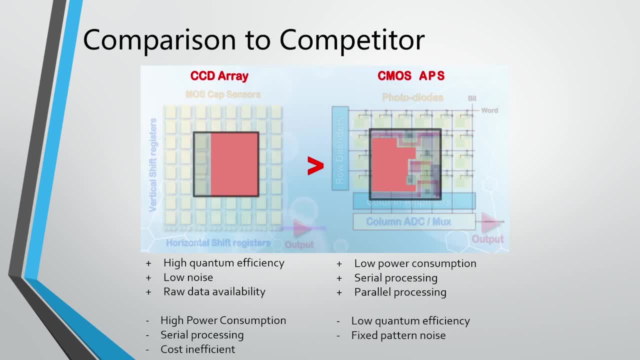 Lastly, CCD array is also cost inefficient because besides the CCD modules we also have to have the clock generation circuit and the signal processing circuit, and they are built with CMOS technology. So we need to have different chips. that works together, But in CMOS they can all be. 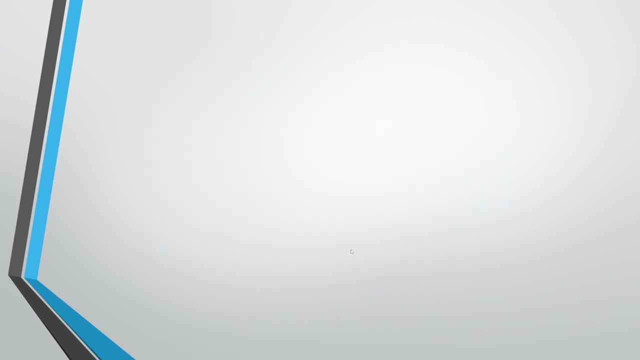 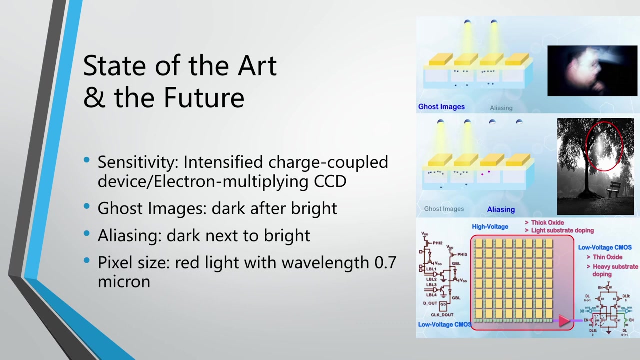 used for one single chip and that reduced the cost hugely. Right now there are still some limitation on CCD. There are the minimum light intensity, on-chip signal processing and inefficient transfer of charges In the sensitivity area. PitBall has proposed many other technologies like intensified CCD. 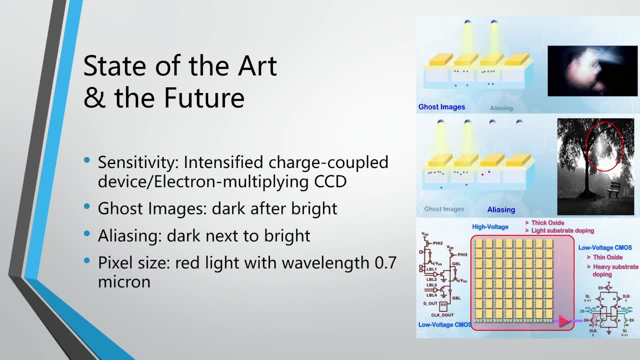 or electron multiplying CCD. They all use similar ideas of multiplying the clarification and caused the noise of the AC sixteen-text cable. They all have similar idea of multiplying the electron or the photon before they get to the CCD device so that even in the dim environment, 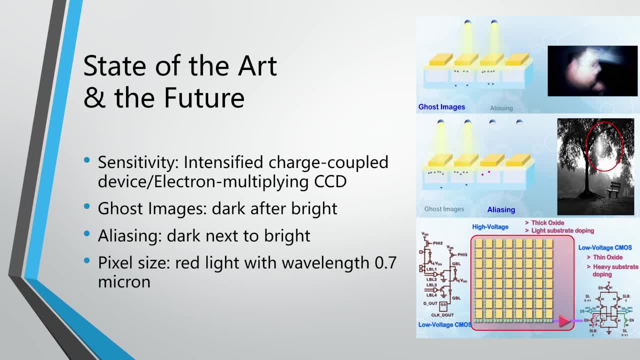 we can still sense something and then. but however, ghost image and aliasing is still very troublesome. ghost image is a dark thing. that is after pricing, and aliasing is a dark thing next to the pricing. we can see on the right. they are both formed because of extra.